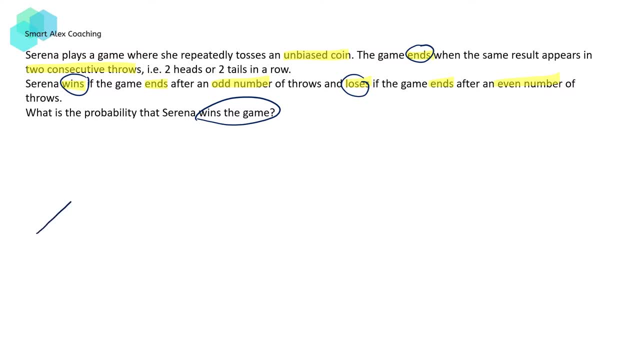 stages of play. Firstly, on your first throw, you can get either head or tail and because this is an unbiased coin, the chance of head is equal to the chance of getting a tail, which is going to be a half. But you can't win after just one throw because there's gonna be no consecutive throws happening. 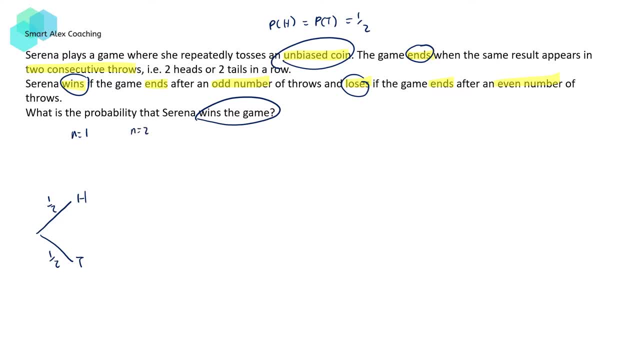 yet. So you're going to move on to your second stage. n is equal to two, So that can branch out to head or tail. Now what's going to happen is, if you get head, then head again, then the game is going to n and you're not going to progress further. You're not going to win, however. 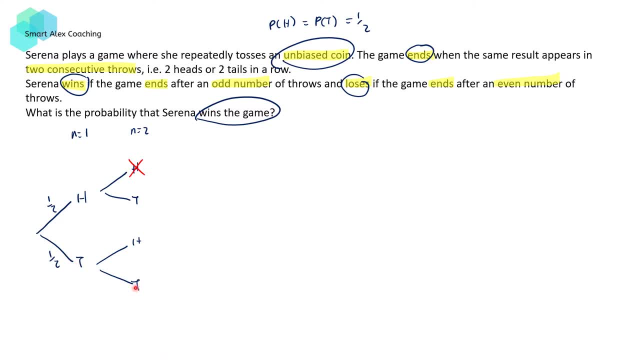 Alternatively, if you get tail, followed by tail, you're also going to lose the game. The game will also end. So I'm just going to cross off to indicate that the game cannot proceed further. So, in order for the game to proceed further, n is equal to two, I have to Dollars and i'm going to 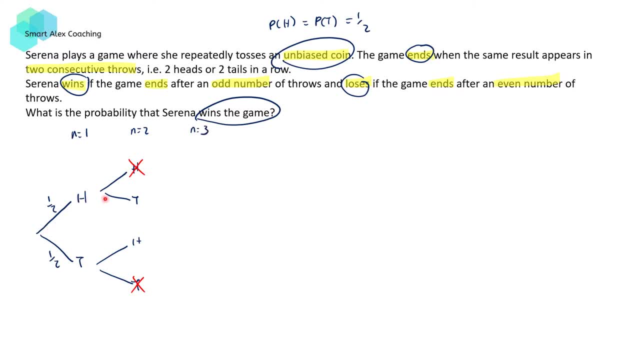 is equal to three. we have to come down this path- head, tail or tail, head- and from these two paths it can progress to head or tail, head or tail, and what we see here is that there are two scenarios in which we can win. the first is if we get head, followed by tail, tail or tail, head, head. so i'm 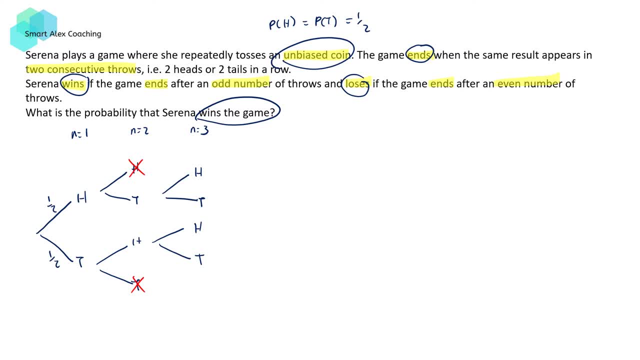 going to like. highlight these two paths in yellow. this is one way of the game winning: after three throws, or this: after we get those consecutive throws, the game ends. those branches will not proceed further, so i'm just going to cross off to indicate that the game ends. however, 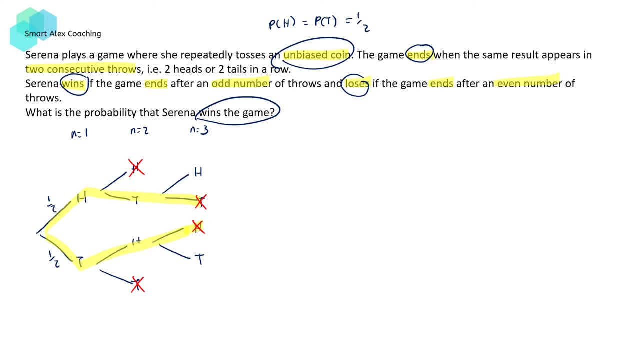 we win the game right, and so the chance of winning the game after three throws is going to be given by a half time times a half times a half, or a half times a half times a half. so the chance of winning after three throws is going to be two times a half cube and we can progress further onto the next stage. 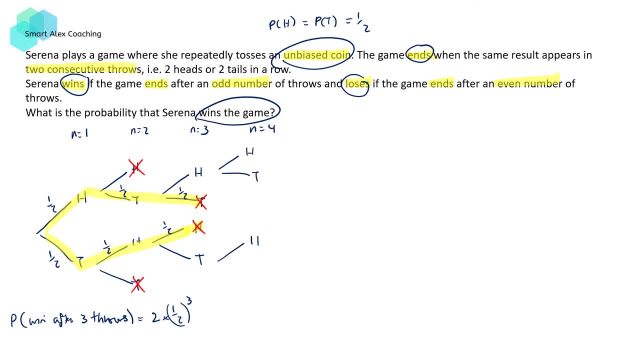 so we can get head or tail, head or tail, and what you're going to see here is that when we get head- head here, the game will end, but we lose the game. so i'm going to cross off that path, same as if we were to get tail, tail right after even number of throws, the game will end. 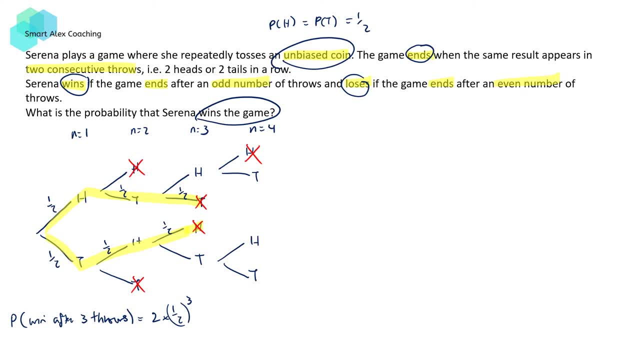 but we lose the game. so i'm also going to cross off this path as well in order to move on to stage five. we can come down by this path- head or tail, head or tail- and in order to win, we have to come via this path. that's going to be one path of winning. alternatively, 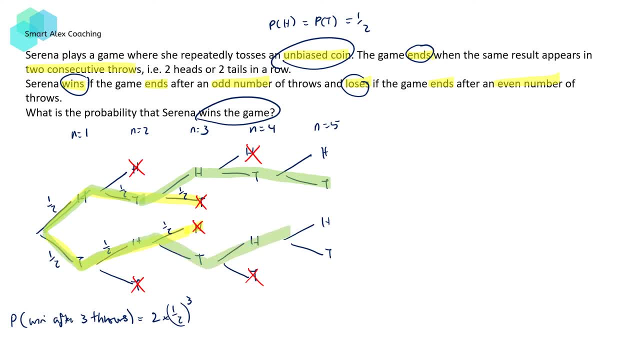 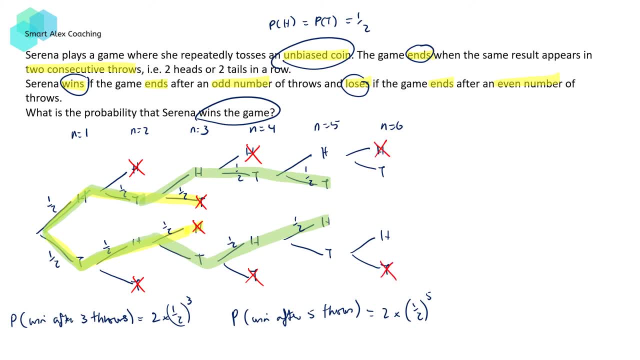 will end here, because we get two consecutive heads, or here we get two consecutive tails, but we can progress on to stage seven. n is equal to seven by this path- head or tail, head or tail- and here we've got chance of winning again. so, in order to win, we this time may be coming down. 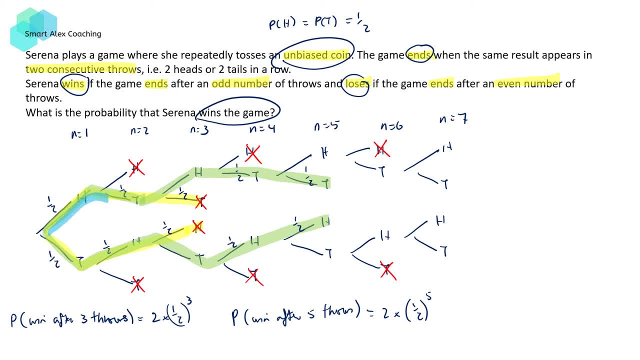 this path. so we've got this path in which we can come down, or we can come down by this path. so the chance of winning after seven throws is going to be given by two times a half to the power of seven, and obviously we can continue this pattern. 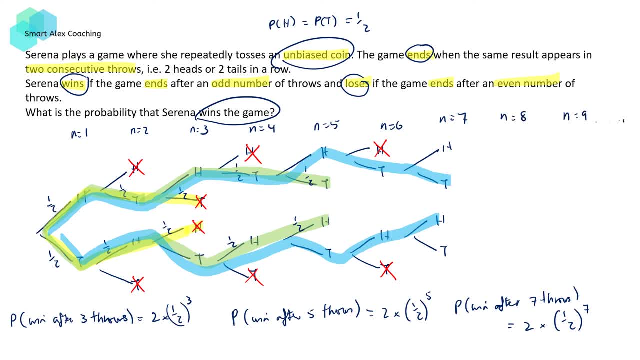 n is equal to eight, n is equivalent, so on and so on, but we're now beginning to see the pattern that's emerging. so if we look carefully, what we see is that after three, three throws, the chance of winning is given by two times a half to the power of three. 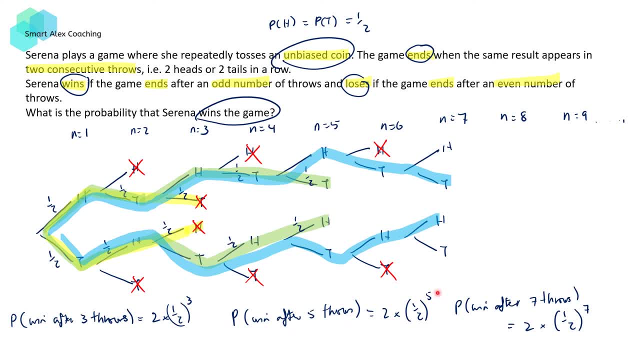 the chance of winning after five throws is two times a half to the power of five. chance of winning after seven throws is two times a half to the power of seven. so you can see the connection there. three throws- power of three. five throws- power of five. seven throws- power of seven. 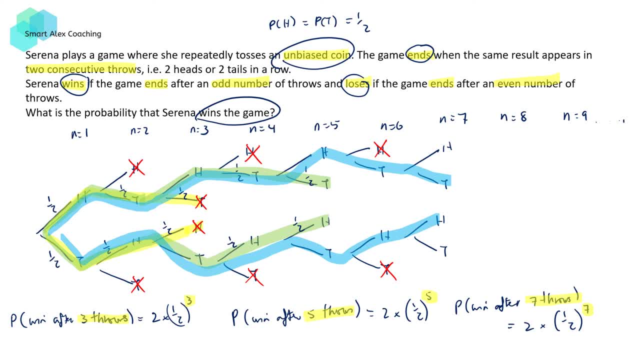 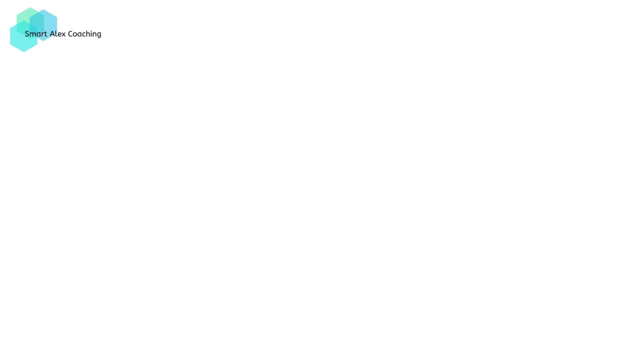 and this keeps on going and it's going to be the basis of our geometric sum. Since Serena will only win the game if she gets consecutive throws. after an odd number of throws, the probability for her to win the game will be equal to the probability of 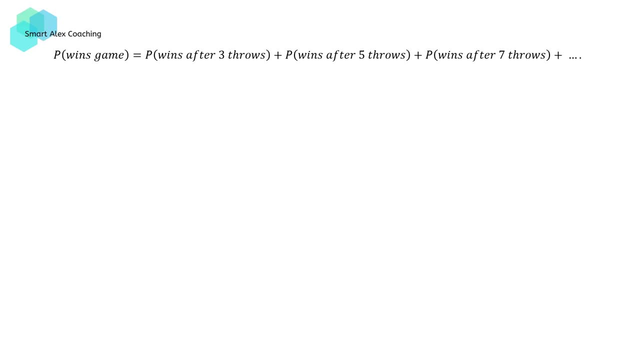 her winning after three throws, plus the probability of her winning after five throws, plus the probability of her winning after seven throws, so on and so on. From the previous slide we've worked out each of these probabilities, so the probability of her winning the game is going. 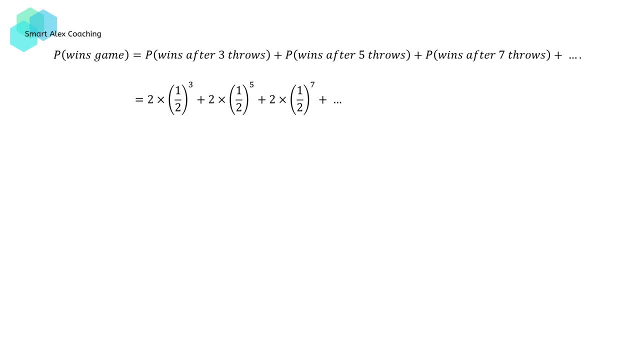 to be equal to two times a half cube, plus two times a half to the power five, plus two times a half to the power seven, so on and so on. We can factorize out the two times a half cube and inside the bracket, what we have is a geometric series. This geometric series has 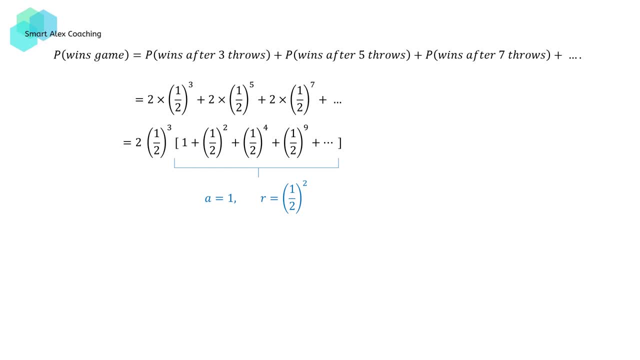 got the leading term: a is equal to one with the common ratio r is equal to a half square. Since the common ratio r is between zero and one, this is going to produce a limiting sum, And recall that the limiting sum is given by: